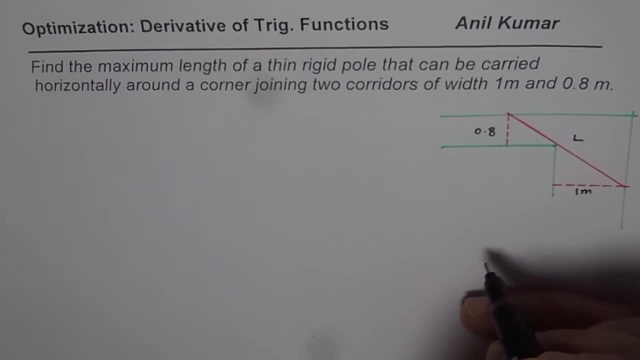 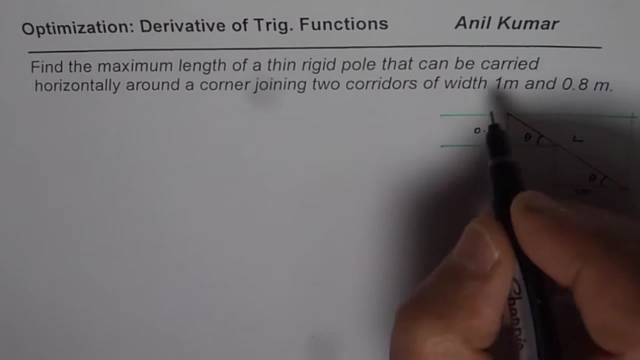 these corridors, right, the maximum length. Now, what we can say is that let the angle be theta. So let us consider. Let us consider this angle to be theta. In that case, length of this rod could be written as: let me. 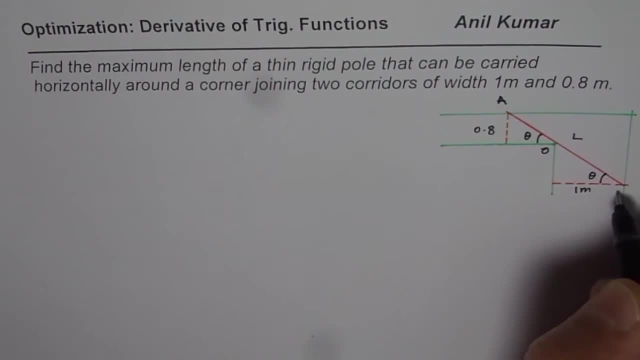 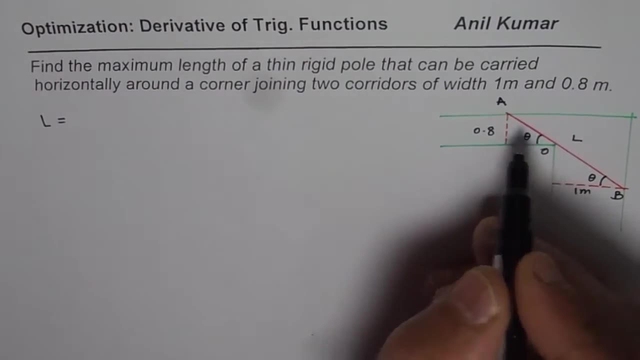 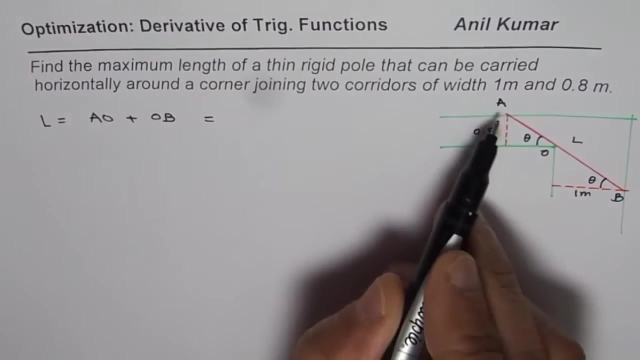 name these points as A, let it be O and B, right, So in that case length L can be written as AO plus OB. Now, from here, AO is: if this is angle, theta, that is, opposite side, is 0.8,. 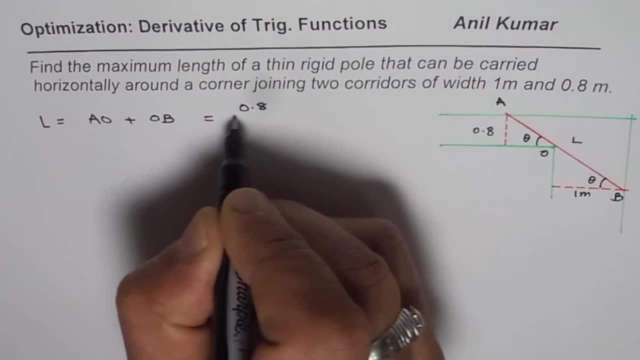 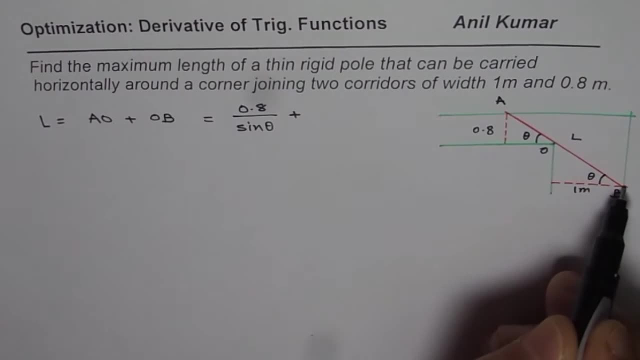 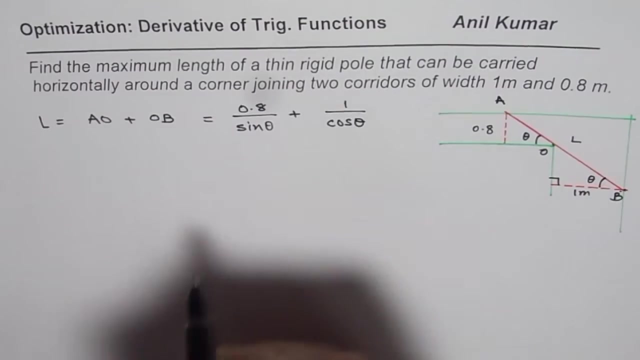 so AO will be 0.8 over sine theta plus OB. the adjacent side is 1 meter and therefore OB will be, which is the hypotenuse, will be 1 over cos of theta. So in this fashion we can get length of the rod or the. 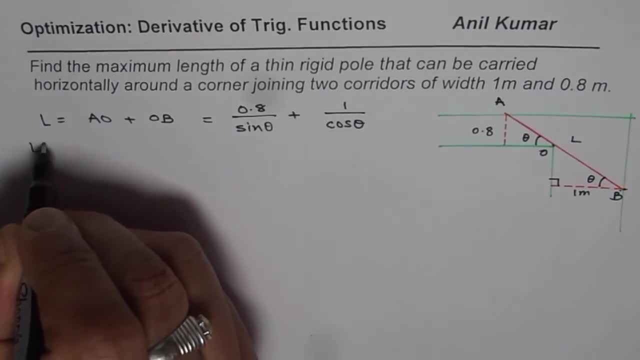 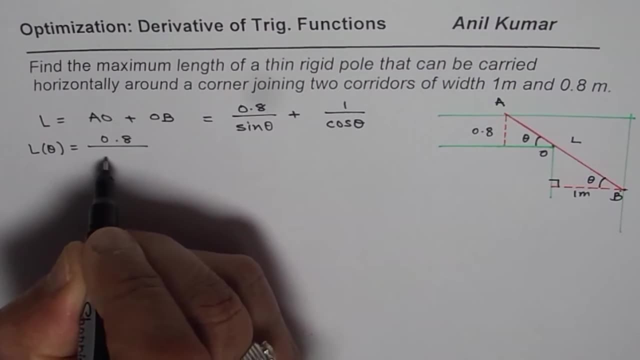 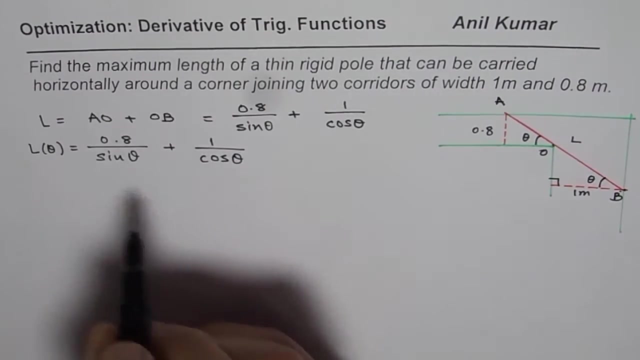 pole in terms of angle theta. So we get function length as a function of angle theta. So which is 0.8 over sine theta plus 1 over cos theta. Now to find the maximum length, what we can do is we can find: 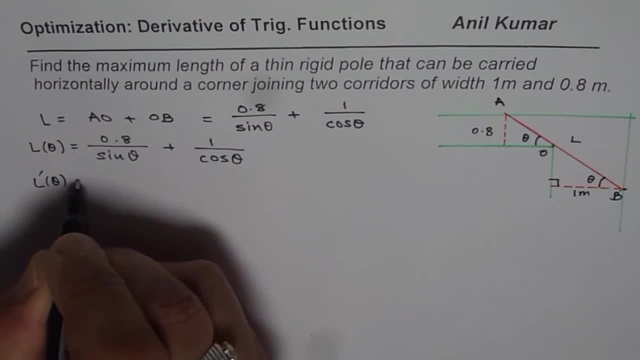 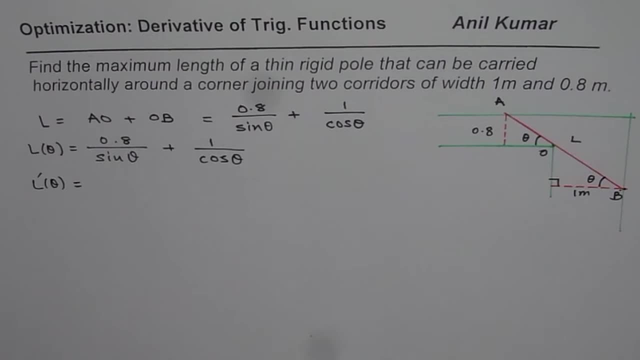 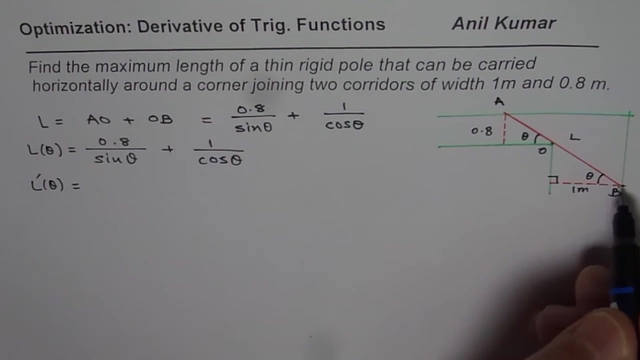 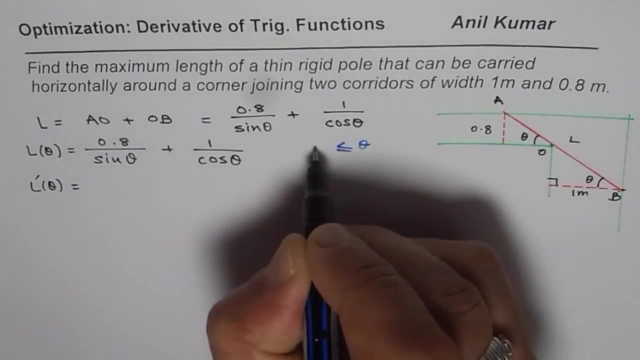 derivative of this function. So derivative will give us the critical points And then we'll also analyze the boundary conditions. Now let us see what are the boundary conditions for us. Angle theta could be either 0 or 90 degrees right. So that is, these are the two possibilities of the angle right. So we have theta which could be greater than 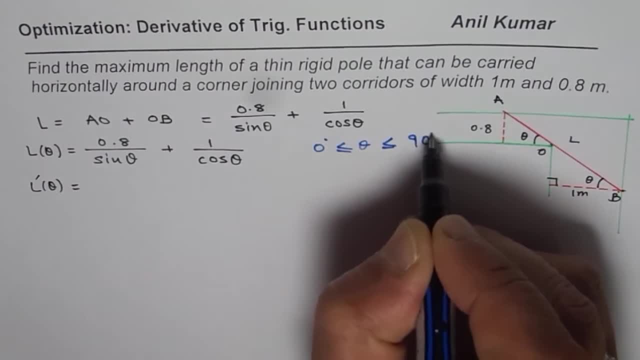 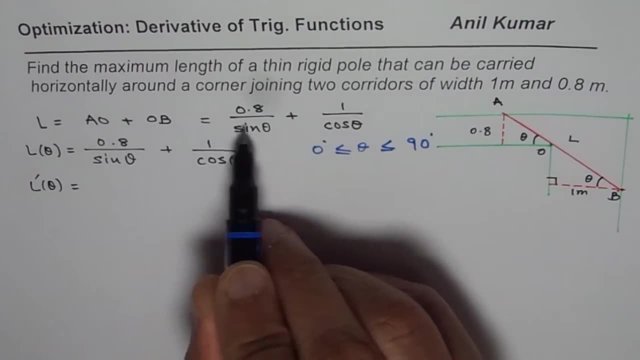 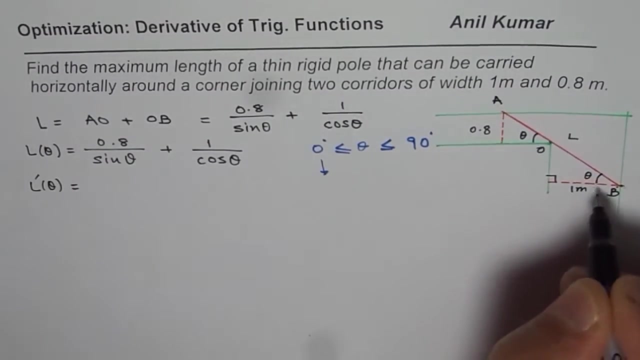 or equal to 0 degrees, or less than or equal to 90 degrees. Now, if I now for 0 degrees and 90 degrees, this equation is not really valid. It, for 0 degrees, theta is 0, then in that case maximum length will be equal to 1 meter. right, If it is flat, then you can. 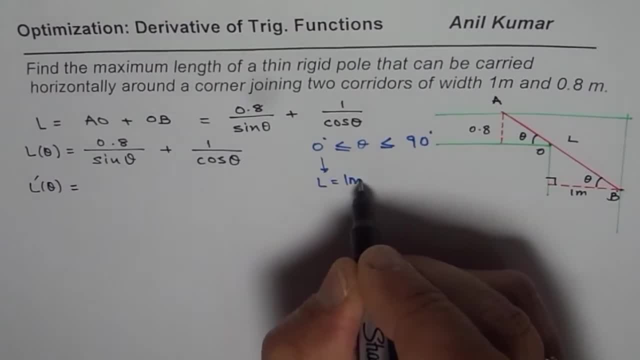 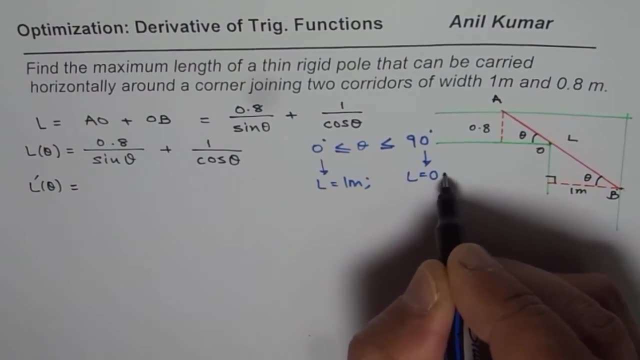 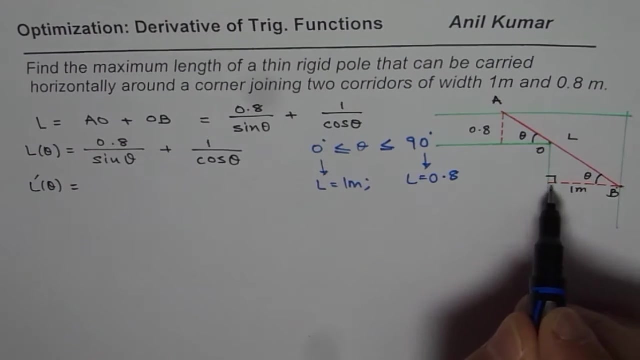 only take that much y, So it is 1 meter. and for 90 degrees, length will be equal to 0.8 meters, 0.8 degrees, right? So that is the length for these boundary conditions in this particular case. right, If it is 0 degrees? 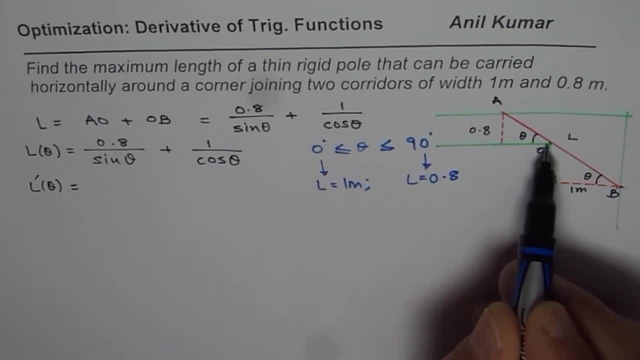 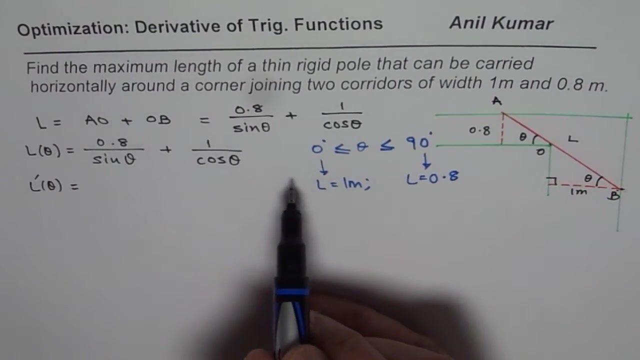 then the maximum length will be 1 meters, And if this angle is 90 degrees, in that case the maximum length will be 0.8 meters, as you can see. So we'll analyze the critical value. If it is more than these, then we'll have a maximum in between. 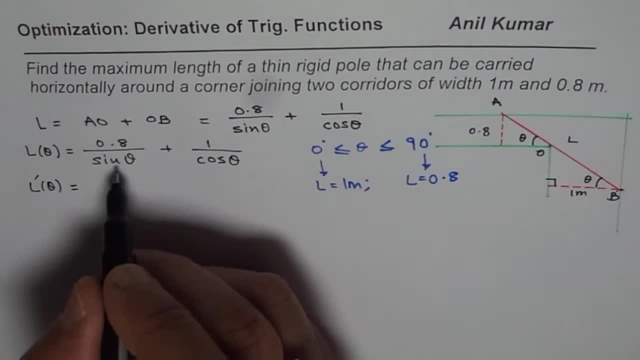 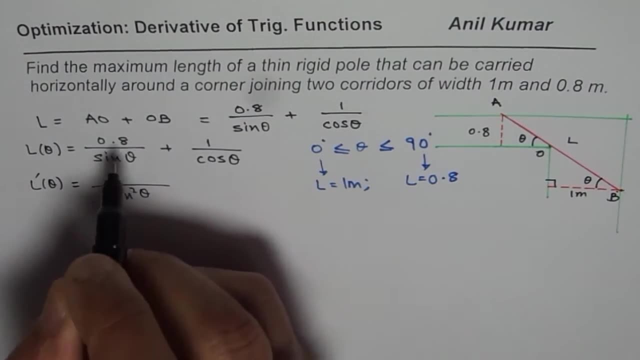 So let's find the derivative of this function. We can apply the quotient rule So it will be sine square theta in the denominator. Derivative of 0.8 is 0. So we get 0 minus 0.8 times derivative of sine theta, which is 0.8 cosine theta. 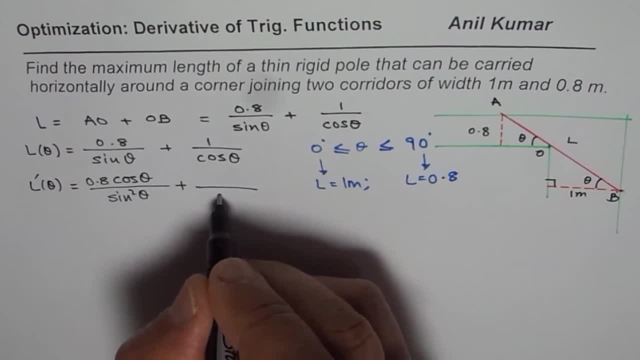 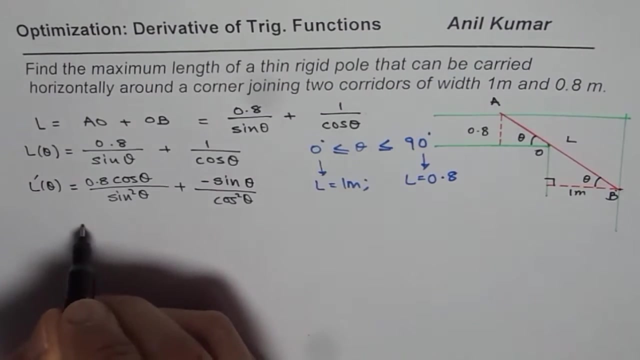 Plus derivative of 1 over cos theta, Cos square theta, We'll apply the quotient rule. Derivative of 1 is 0.. So minus 1 times cos theta derivative, which is minus sine theta. Now let's take the common denominator, which is sine square theta. 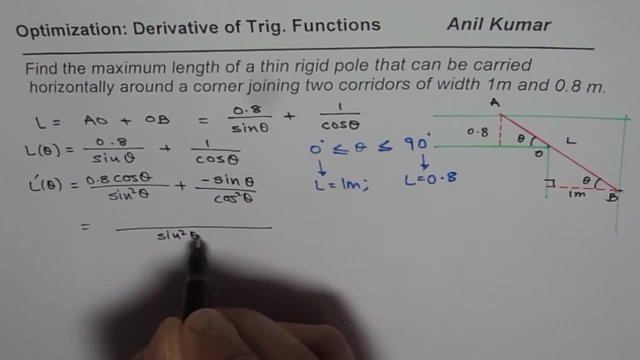 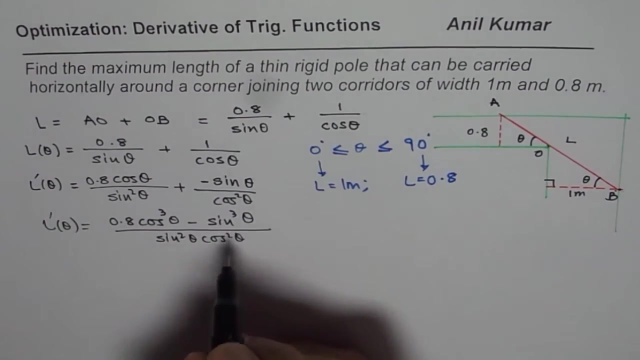 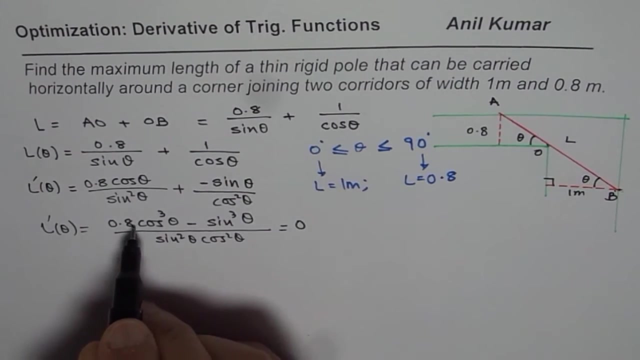 Cos square theta Cross multiplies, we get 0.8 cos cube theta minus sine cube theta. So that is the derivative for the ladder. Now for critical number. this derivative should be equal to 0.. That being 0 means the numerator should be 0, correct. 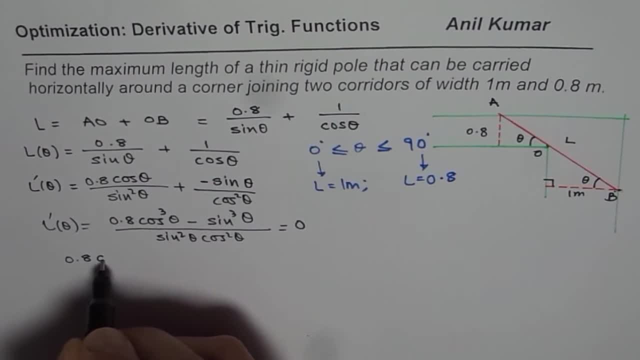 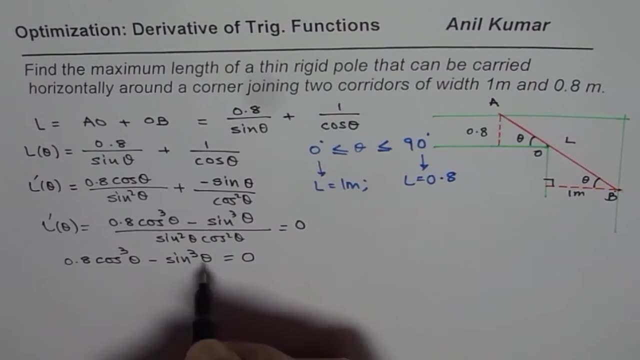 So the numerator is 0 means 0.8.. Cos cube theta minus sine cube theta equals to 0.. So we can now solve taking sine on one side. So we have sine cube theta equals to 0.8. cos cube theta. 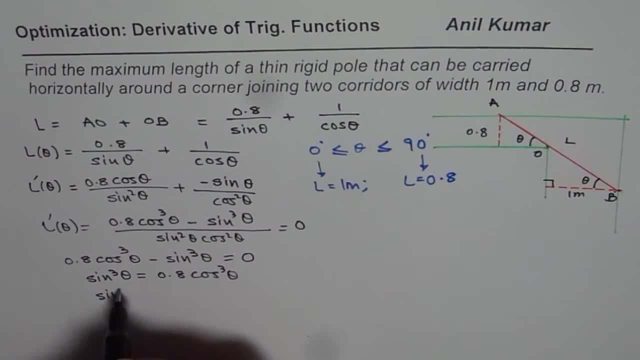 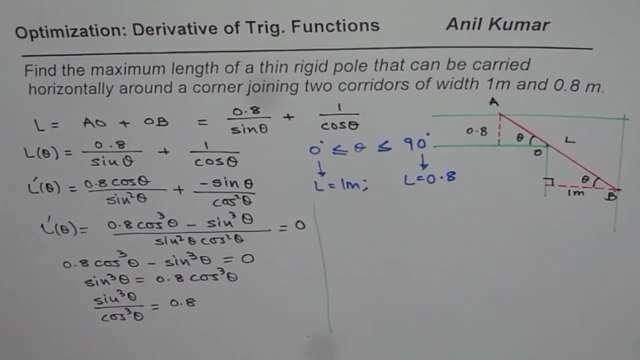 Dividing by cos cube theta we get sine cube theta. divided by cos cube theta equals to 0.8.. So that is tan cube theta, right. So that gives us 0.8.. So that gives us the critical number at let us solve it on this side. 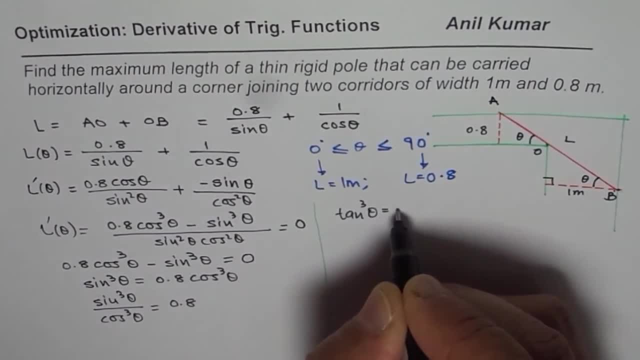 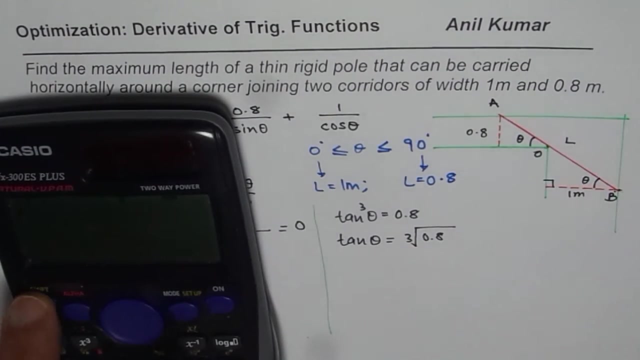 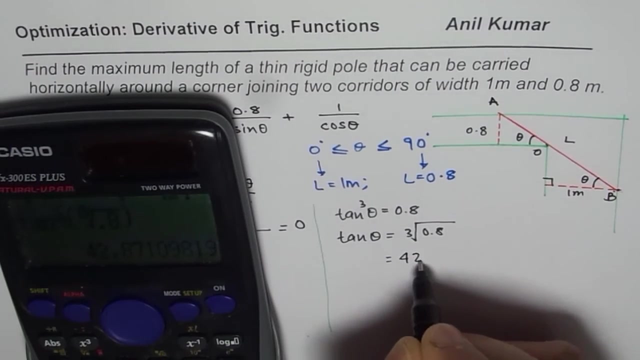 Tan cube theta equals to 0.8, or tan theta equals to cube root of 0.8.. So let us use the calculator to find the answer. So we have shift tan inverse of cube root Of 0.8, which is equal to 42.87 degrees, right. 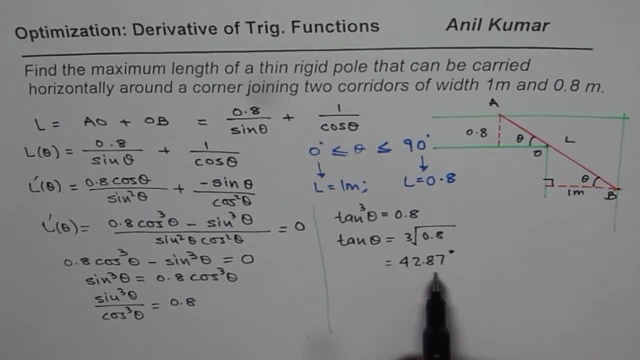 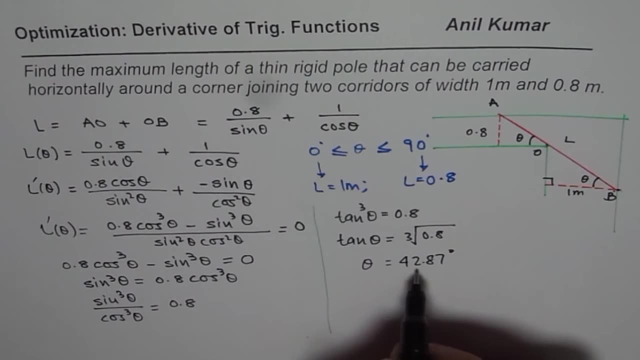 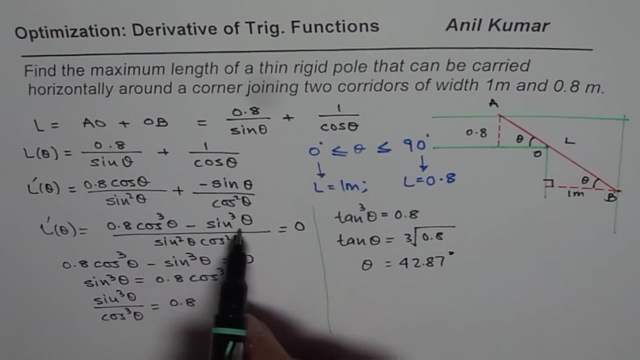 So that is the value of theta, right. So we get theta equals to tan, inverse of this, which is indeed 42.87.. Now what we can do is we can analyze on either side whether the value is changing From negative to positive or not, right? 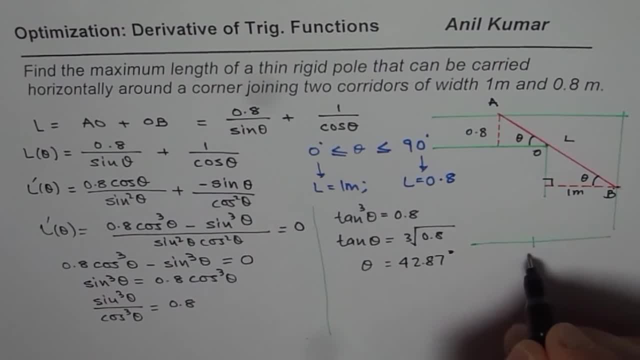 So we will analyze the angle given to us, which is 42.87.. We can take a value of angle which is less than this- let us say 30 degrees- and more than this- let us say 60 degrees- in the given equation. 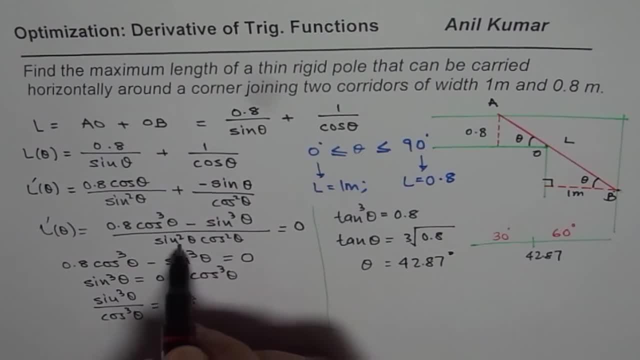 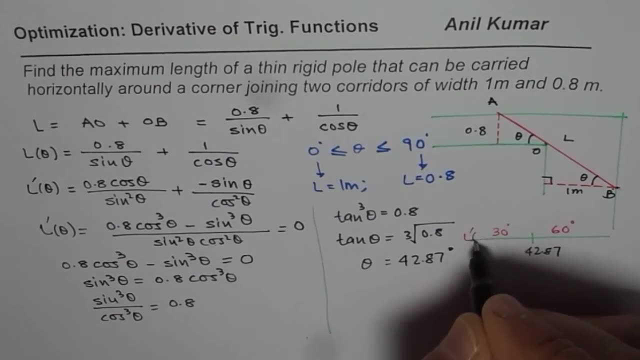 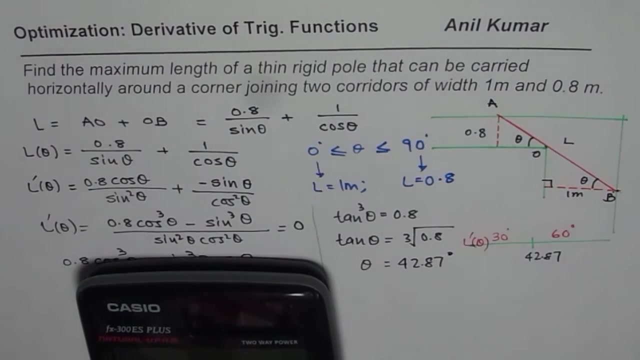 We know numerator is always positive, since they are squares. We will analyze the. I mean denominators are always positive, since they are square, So we will analyze the numerators for the sign. So now let us calculate the numerator for 30 degrees and 60 degrees. 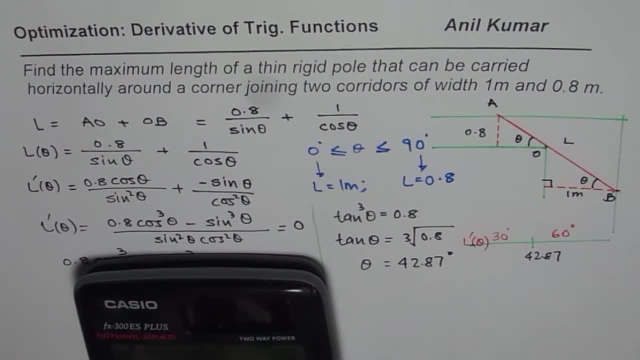 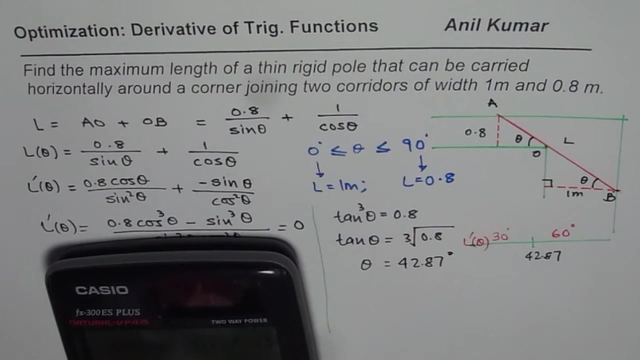 So we have 0.8 times cos cube theta. So 0.8 times within brackets, cos of 30 degrees: Bracket close will cube this Minus Sin cube. So we will put it in brackets. Sin of 30 degrees is equal to it's a negative, approximately in decimals, 0.39 positive. 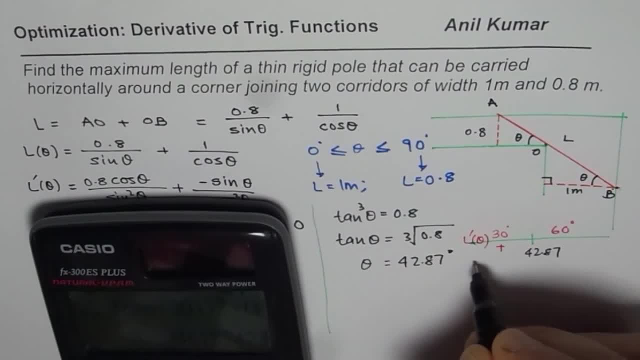 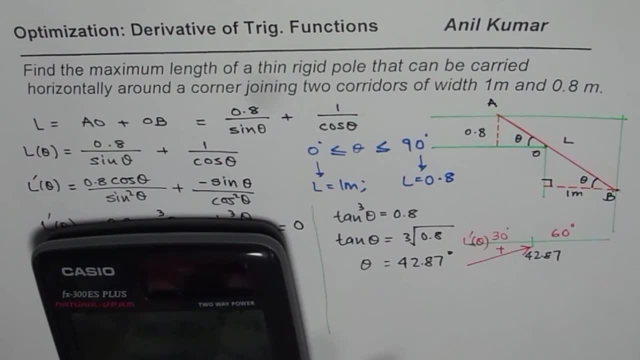 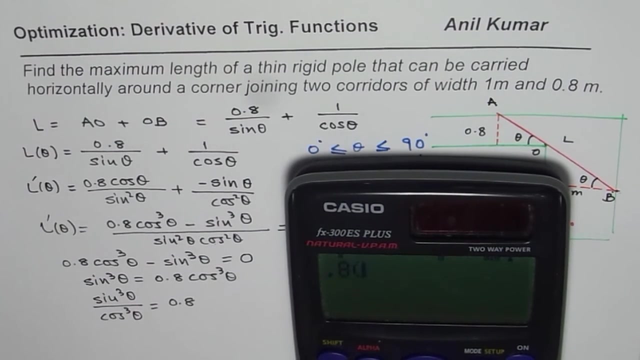 So it is a positive value of 0.39.. 0.39 means that the derivative is increasing or the function is increasing. Now let us substitute 60.. So if I use 60 here, then what do we get? We get 0.8,, within brackets, cos of 60 degrees. whole cube.